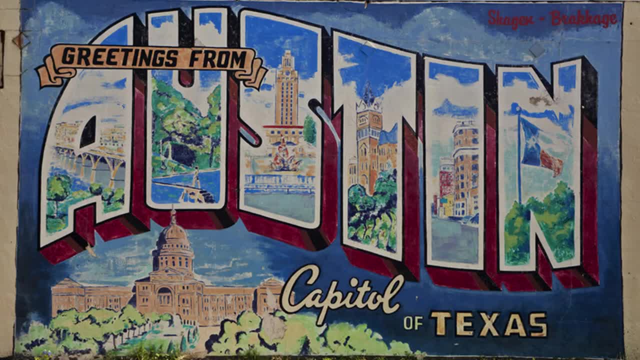 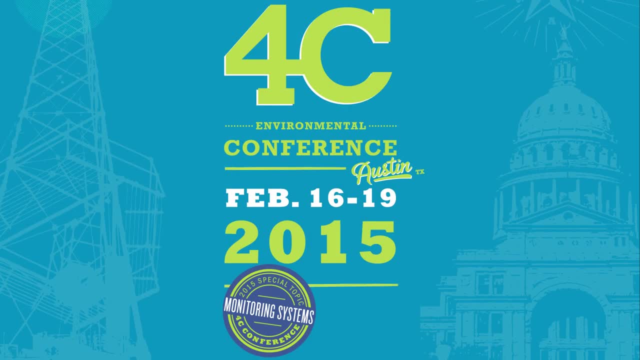 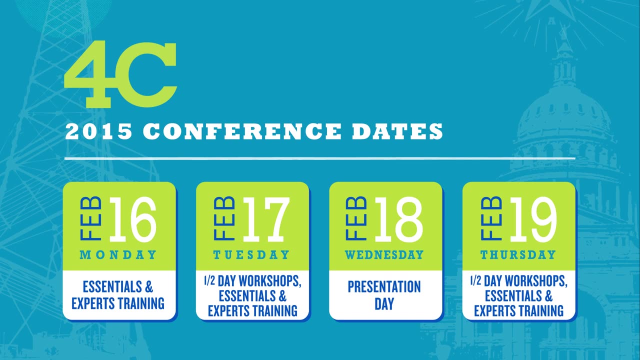 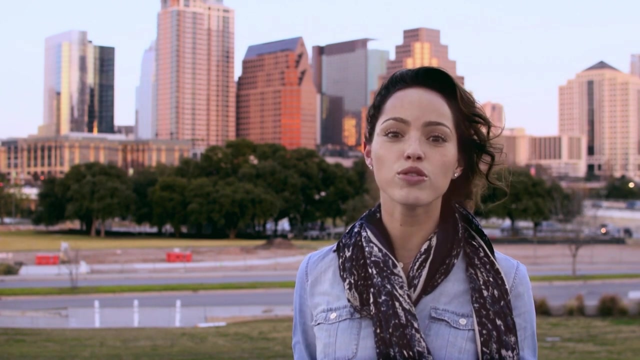 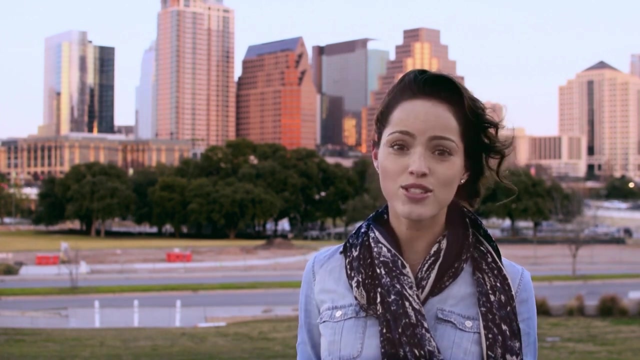 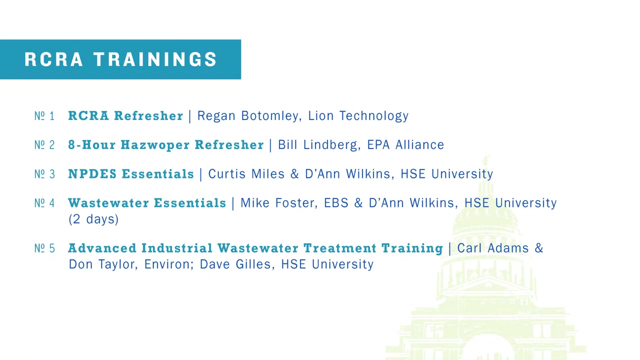 Changing times mean that the 4C Environmental Conference agenda keeps expanding to accommodate new regulatory initiatives and topics. This year we have an even larger selection of trainings, presentations and social events. so that you can make the most out of your time here in Austin. Our agenda features a number of expert-led 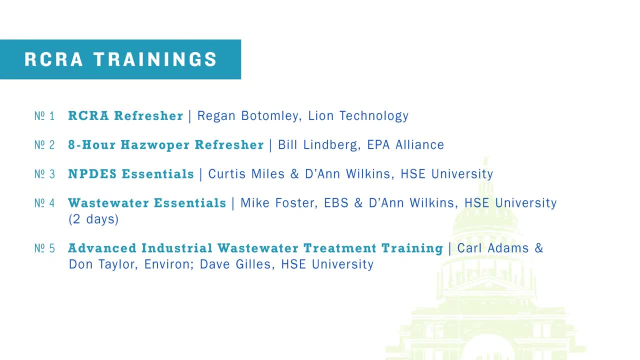 trainings by various vendors and partners. Our record refresher training will help you fulfill your annual training requirements. Our National Pollutant Discharge Elimination System Essentials course, or NPDES Essentials, can be combined with our SPCC and Stormwater Compliance Manager training for those who are responsible for managing developing 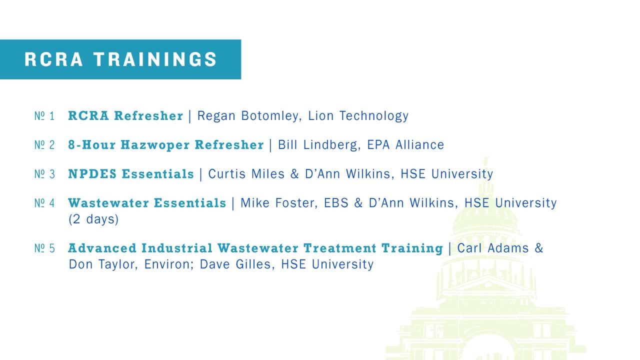 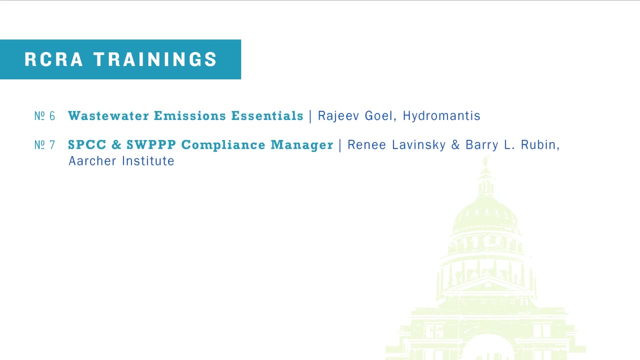 and implementing these plans at their facility. Wastewater courses will support personnel involved in the operation and oversight of wastewater treatment activities, including industrial activated sludge systems, source characterization and control, biomonitoring or wet testing technology, evaluation and selection. or hear the latest on Zero Waste. 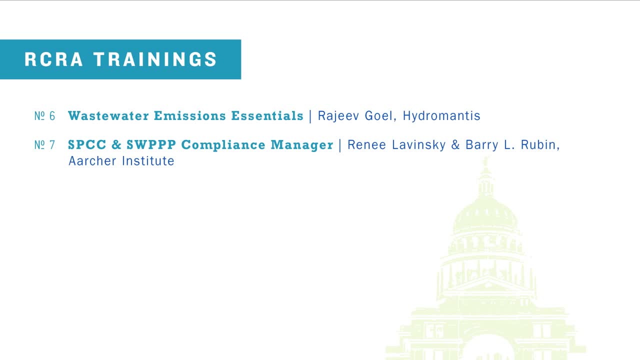 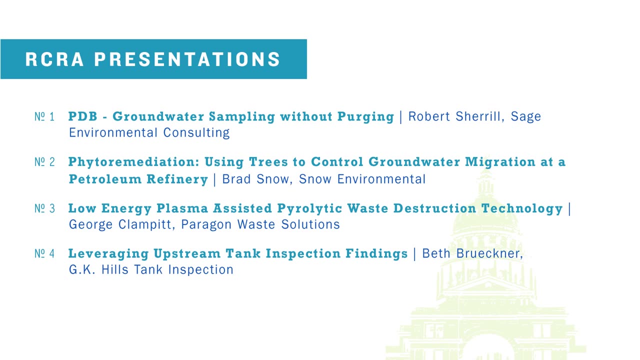 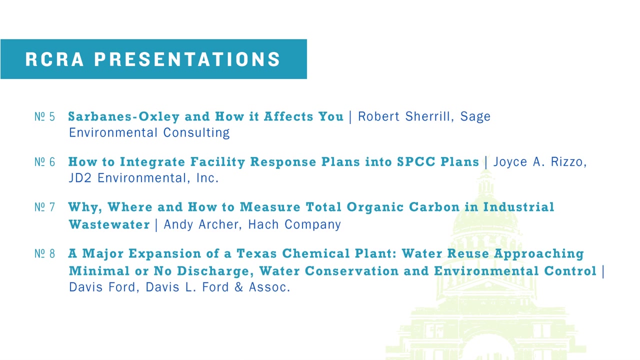 Discharge or VOC, Biotreat and industrial water reuse and recycle. The 4C team is constantly looking for presentations that are applicable to you and your facility. This year's agenda features presentations by Andy Archer of HACC on the why, where and how to measure total. 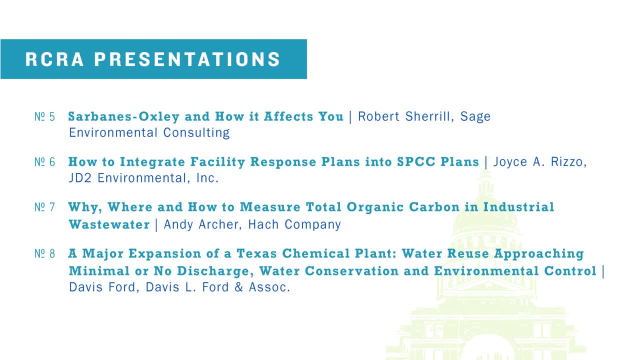 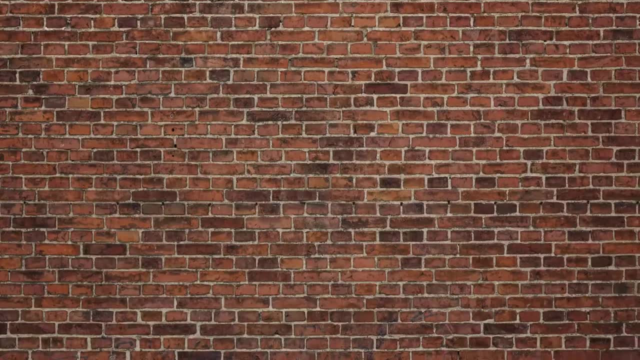 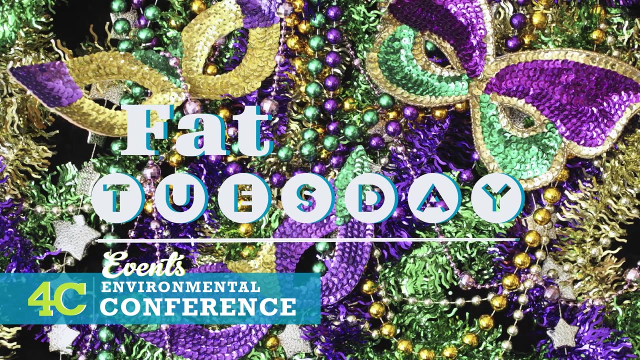 organic carbon in industrial wastewater. Make the most out of your time here at 4C, From a movie screening of the film Frack Nation to a Fat Tuesday celebrations or a roaring good time at our speakeasy casino night. we have so much more to offer. For more information. 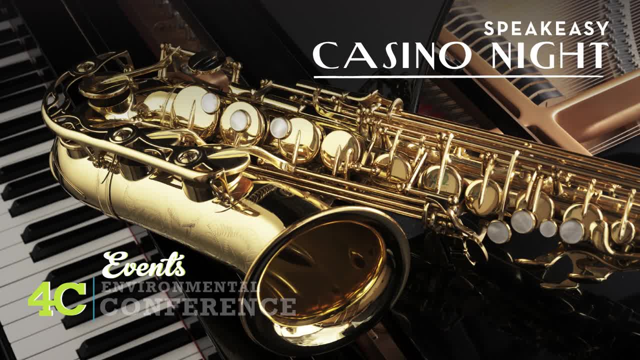 we have something in store for everybody: to sit back, relax and meet industry leaders, Call one out to collaborate and connect with peers and contribute to industry compliance. See you in Austin.